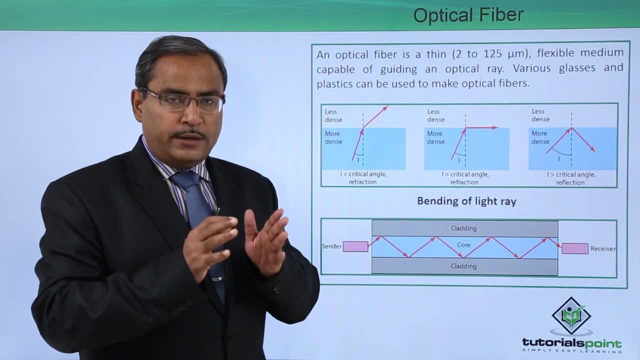 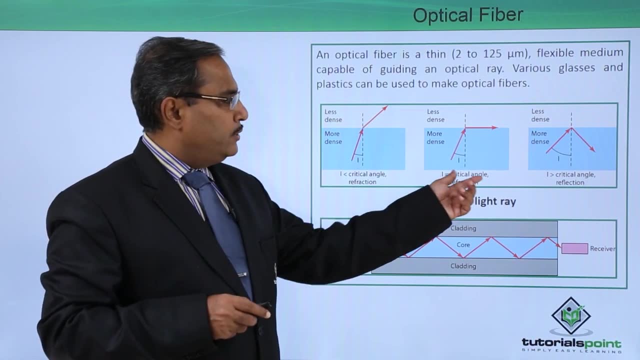 just glancing at the surface in between the denser and the rarer media. So this is the angle of incidence. So that is, I is equal to. that is, angle of incidence is equal to critical angle. there is a refraction here. So now, here you see, if the angle of incidence 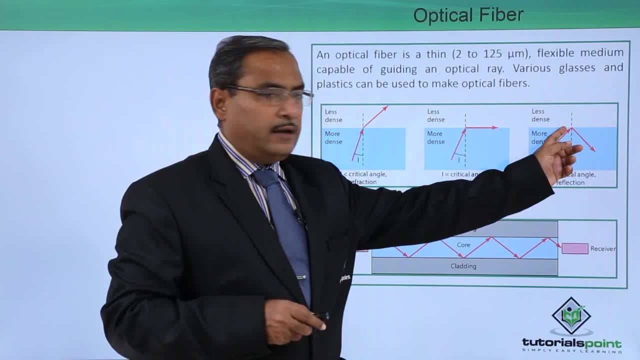 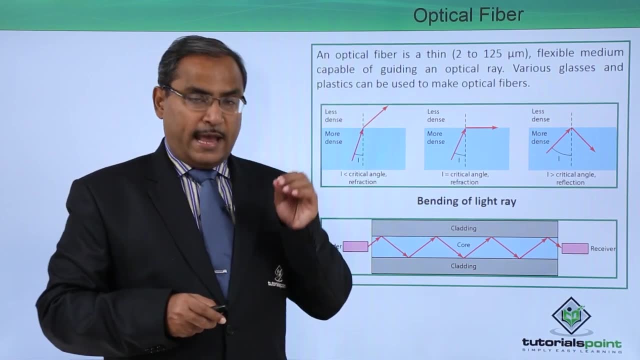 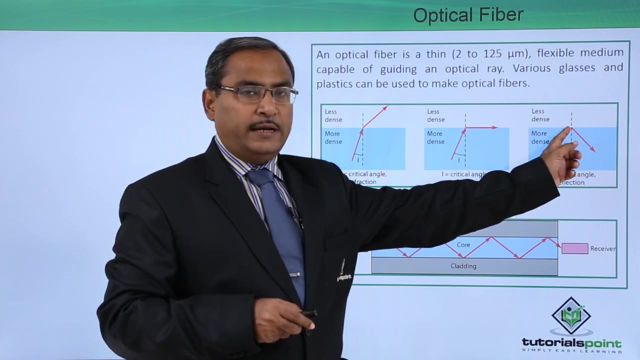 is greater than the critical angle, then in that case the refracted light will not go to the lighter medium. then the interfacing surface in between the two media will behave as a reflector And the ray of light will be after getting reflected instead of getting. 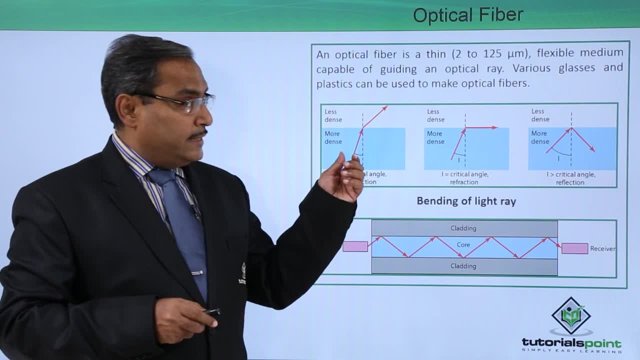 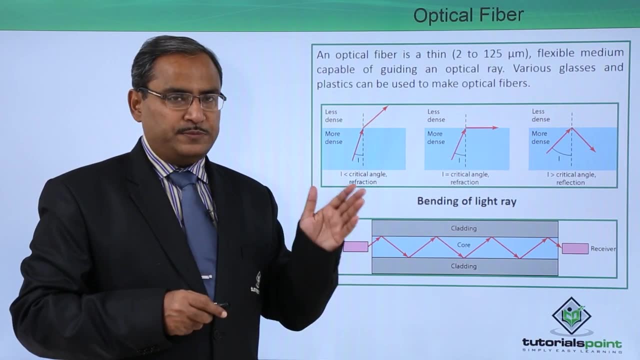 refracted, will be coming back to the denser medium. Thank you, And this is. this is the known as total internal reflection, because no energy will be absorbed at the interfacing surface between the two media. so that is why it is called total internal. 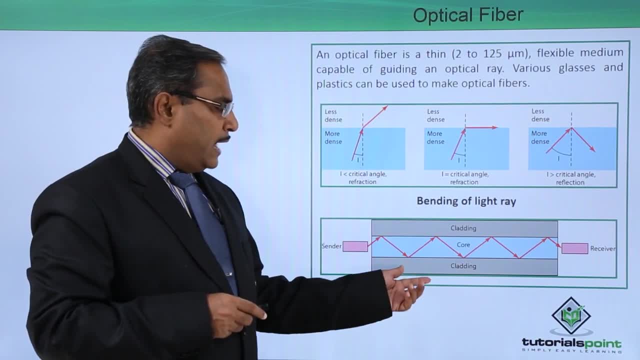 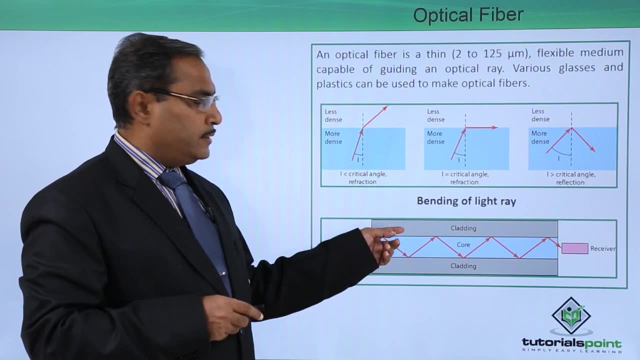 reflection. So now, if we consider the bending of light here, you can see this is our center and this is our core and this is our cladding. so denser to rarer. So this particular angle of incidence, if it is more than the critical angle, then instead. 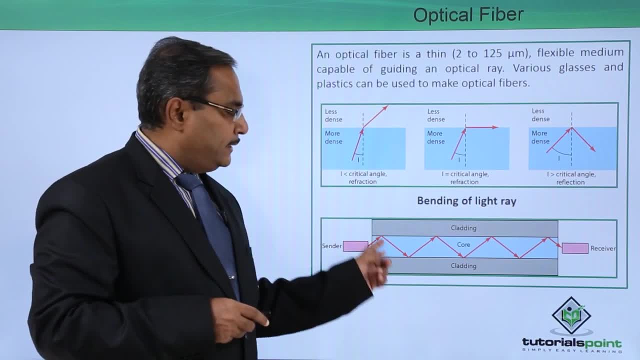 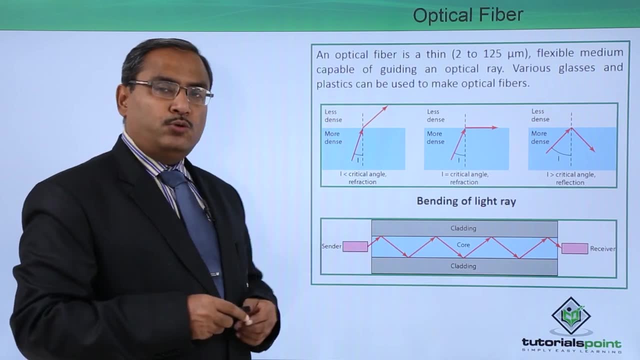 of getting refracted, the ray of light will be reflected back, and in this way the reflection will take place for multiple number of times. ultimately it will be reaching to the receiver As it is taking total internal reflection, so energy loss will be almost negligible here. 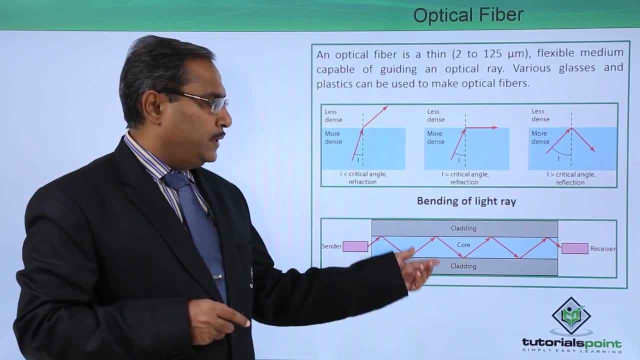 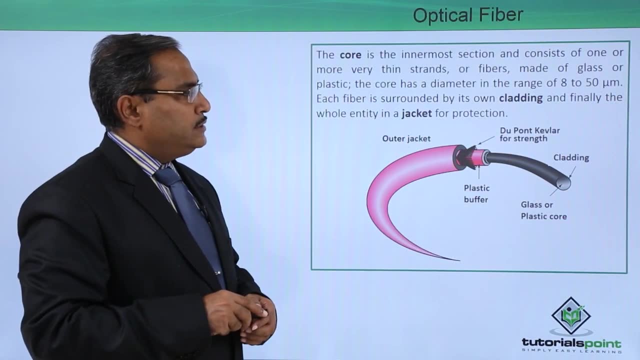 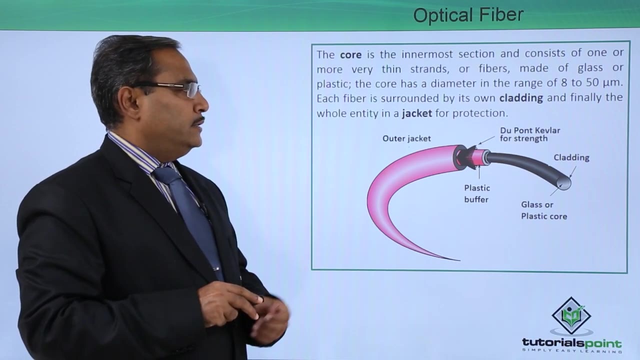 so that is why it is called the. this is the basic principle of this optical fiber and it is called the bending of light ray. The core is the innermost section and consists of one or more very thin strands Or fibers made of glass or plastic. the core has a diameter in the range of eight to fifty. 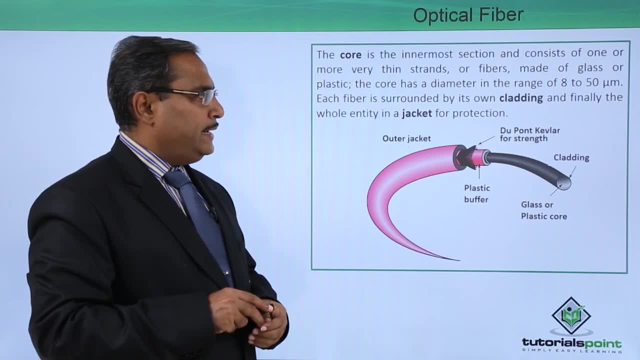 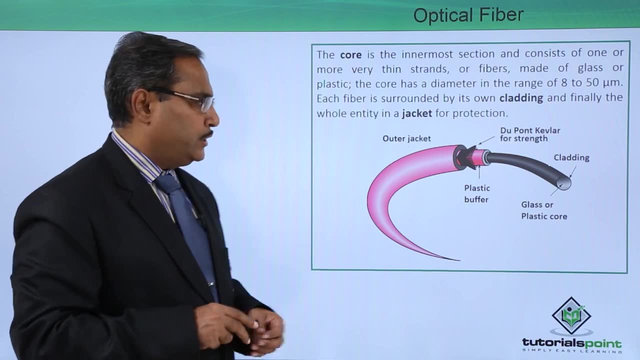 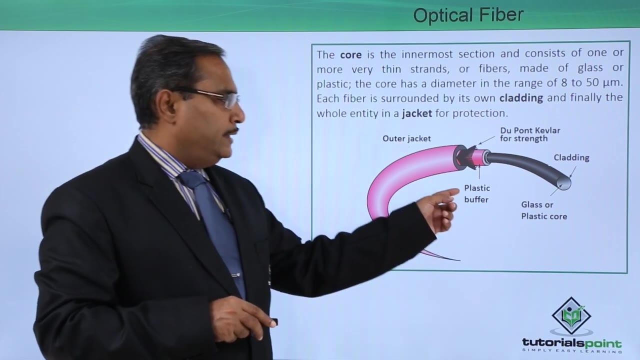 micro meter. each fiber is surrounded by its own cladding and finally the whole entity will be put in one jacket for the protection. So here we are, having the respective cladding and this is our glass or plastic core and this is a plastic buffer. here. 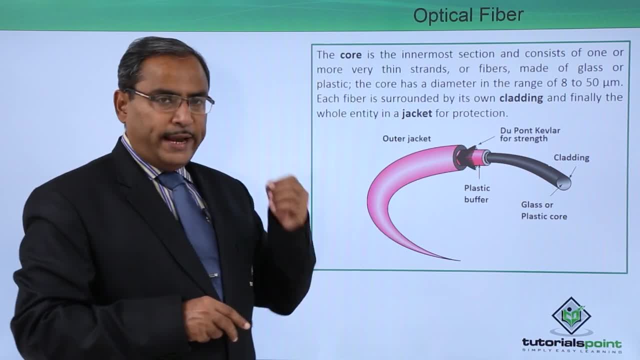 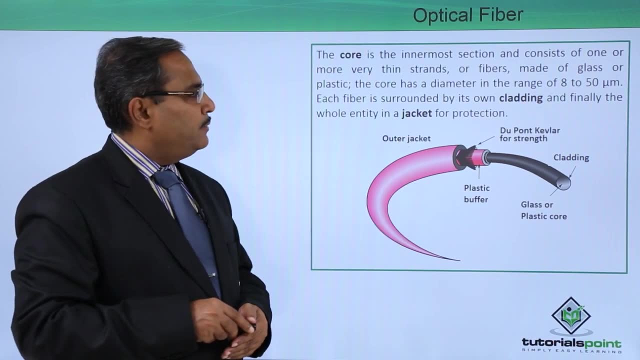 And this is the respective surface waves are there to increase the strength of this optical fiber and it is our outer jacket And that is a construction of this optical fiber. This optical fiber, how this light will be passing through the optical fiber, what are? 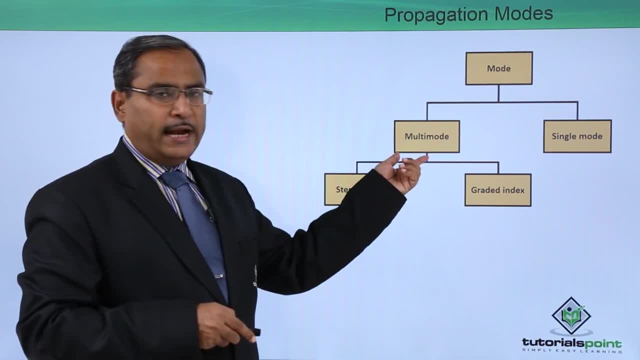 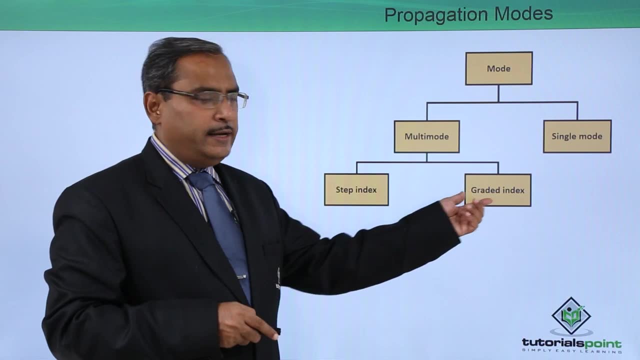 the different modes. So this mode can be categorized in two different categories. One is the multi-mode and the one is the single mode. This multi-mode can be of two types. One is a graded index and the one is a step index. 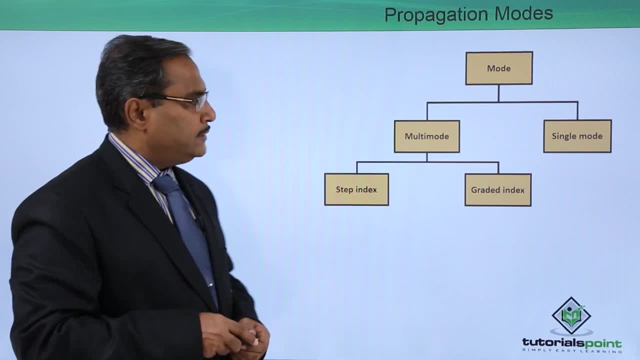 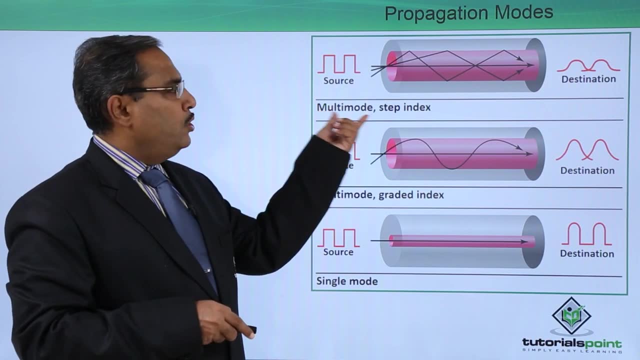 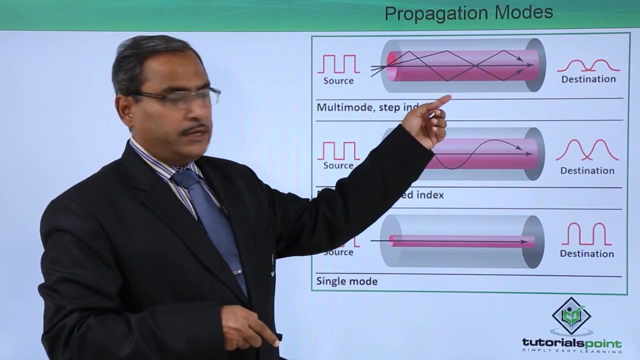 So what is the difference between graded index and step index? we will be discussing that one. Just consider this one. here we are having this multi-mode or step index, So here you can find that multiple rays will be having their reflection at this particular 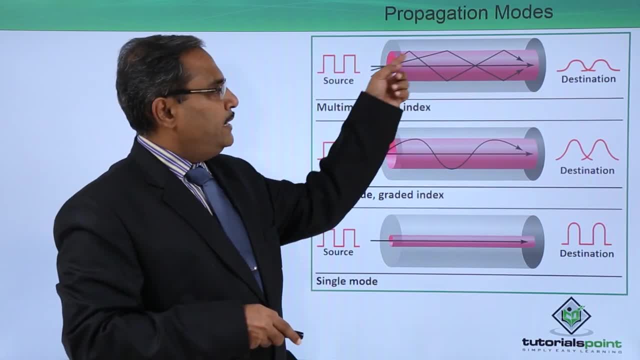 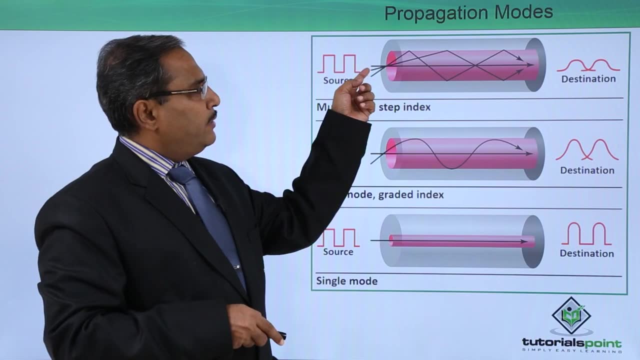 interface between the two media. You can see this ray is having 1,, 2,, 3 times reflection. then it is reaching to the destination. But another ray: you can find That it is having only 2 times reflection. it will be reaching to the destination accordingly. 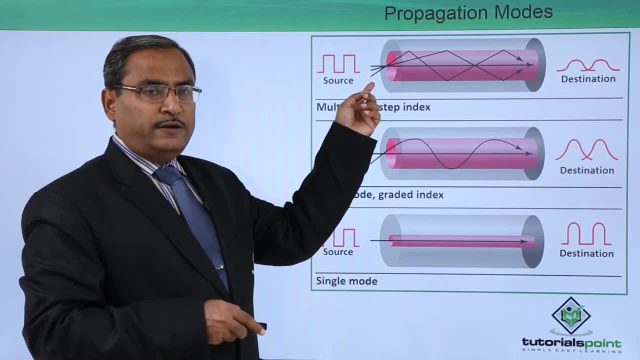 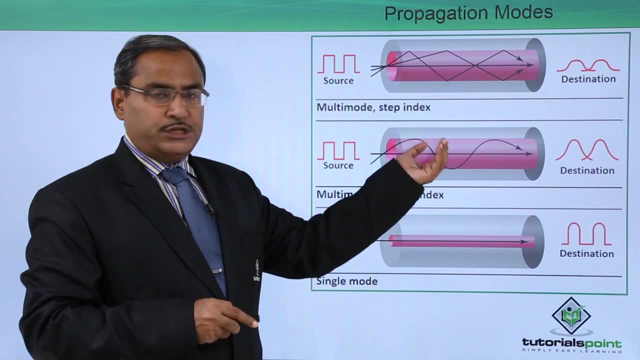 So same ray, that means the multiple rays which will be originated from the same source at the same time, may reach at different time at the destination because they might be suffering different number of reflections. So that is the source and that is our destination. 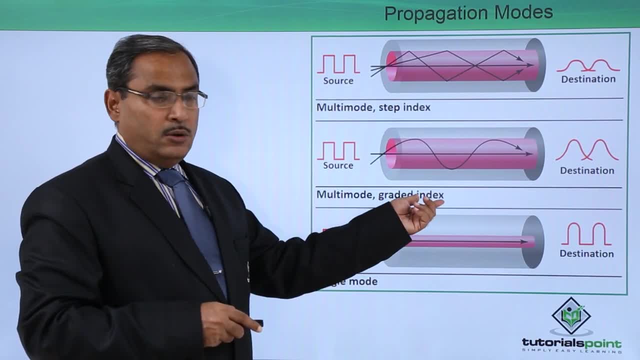 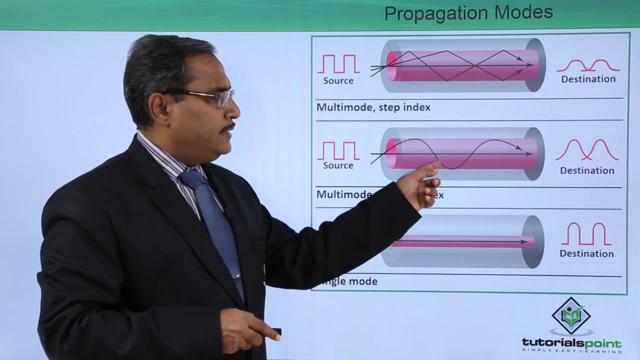 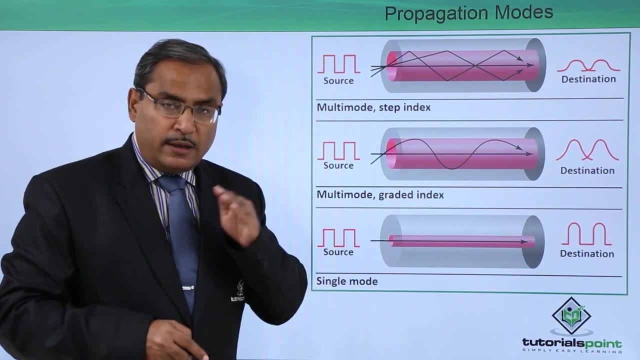 So in case of multi-mode graded index, where this particular density of this core is varying, so as a result of that, this is the ray. the optical ray will be passing through this optical fiber in this particular fashion because the density is varying. 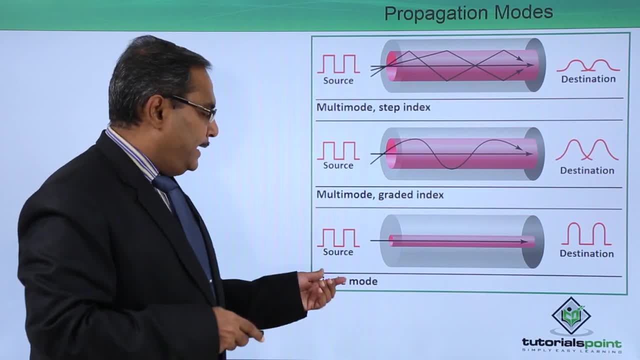 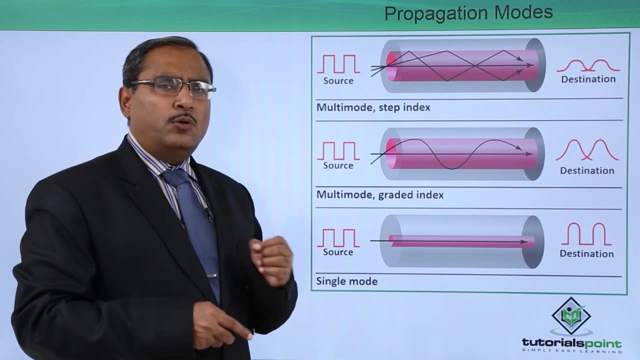 So obviously the refractive index will be also varying. In case of single mode, the dimension of this particular core has become so narrow that it is almost coming the dimension of the frequency of the ray, dimension of the wavelength of the ray. So, as a result of that, if the dimension of this 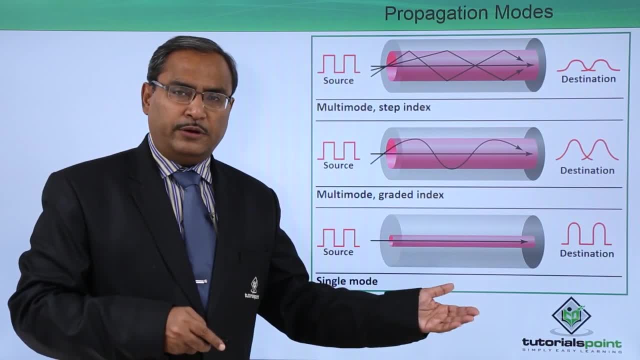